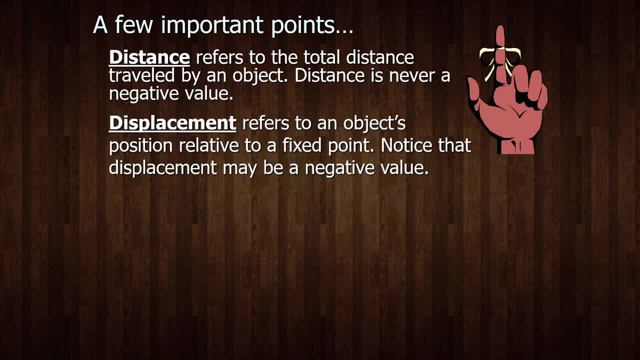 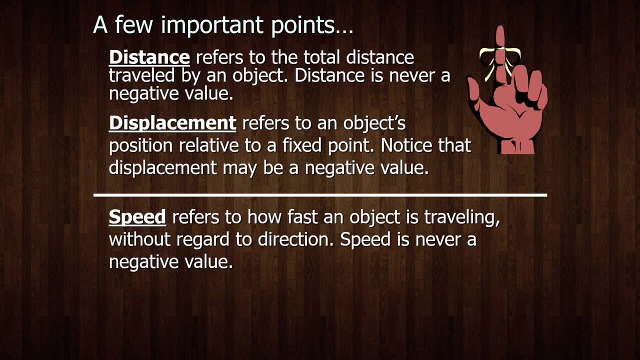 as being the positive direction, and then the opposite direction is the negative direction. Similarly, when we're talking about how distance and displacement are changing, we have a couple of words that we use, The first of which is speed. Now, speed refers to how fast an object is traveling without regard to direction. So if we're talking about a object, that's, 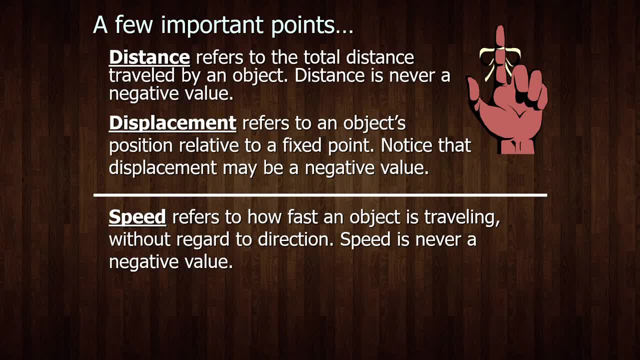 moving at a certain speed. we're talking about speed as a direction. So, since we're not referring to direction when we talk about speed, speed is never given a negative value. Velocity, on the other hand, refers to how fast an object is traveling and the direction of its motion. Now, since we're 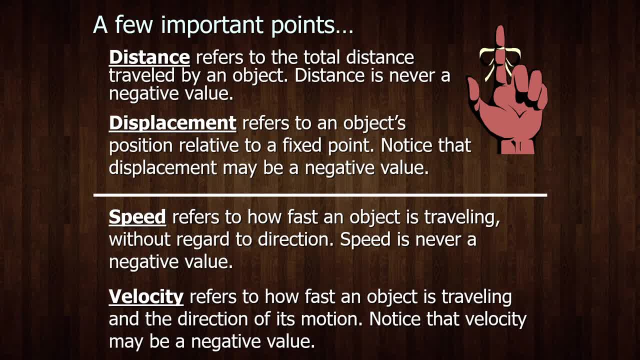 including the direction of motion. here, velocity can be given or described using a negative value And, once again, usually what happens is we have some direction is the positive direction and then the opposite direction to that is the negative direction. So let's do a little example here. 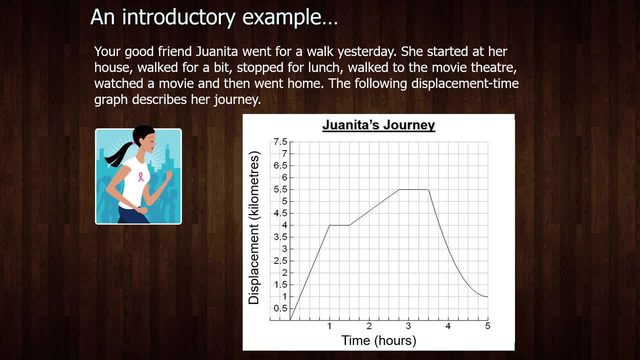 Your good friend Juanita- and perhaps you didn't know you had a good friend Juanita, but you do- and she went for a walk yesterday. She started at her house, walked for a bit, stopped for lunch, walked to the movie theater, watched a movie and then went home And we have a displacement. 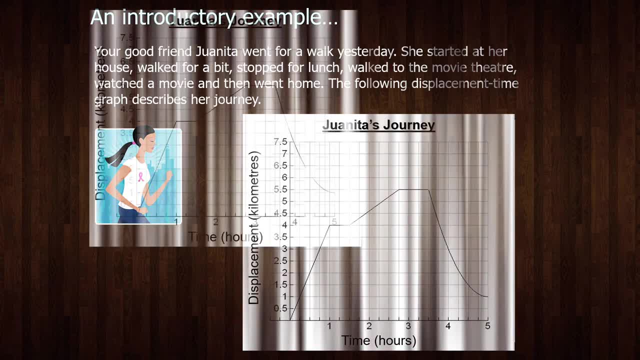 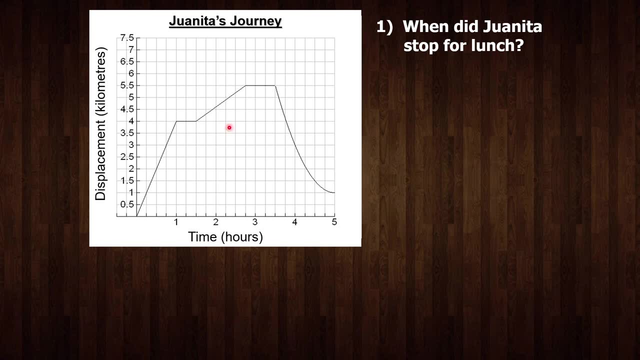 time graph here that describes her journey. So let's ask ourselves some questions about this journey. First of all, when did Juanita stop for lunch? Now, remember, we're measuring displacement on the vertical axis Here and we're measuring time on the horizontal axis, So how can we tell when Juanita stopped for? 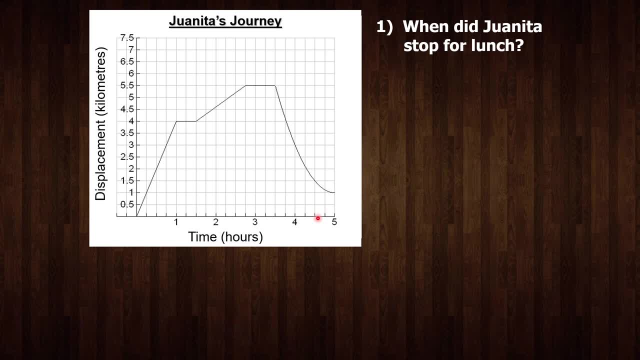 lunch. Well, if she was stopped, her displacement would not be changing. That is, you can think of it as her distance from home would not be changing, Which means for a period of time we should be at the same displacement. Now we see that happens in two places. First of all, here, where we're at, 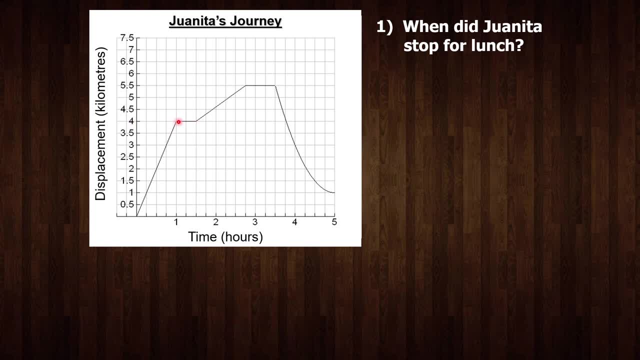 a displacement of four kilometers. And how long is that interval there? Well, notice that four square is one hour. So each of these little squares here is 15 minutes. So this interval here must be 30 minutes or a half an hour. But we also have the same thing happening up here, where we have a 45 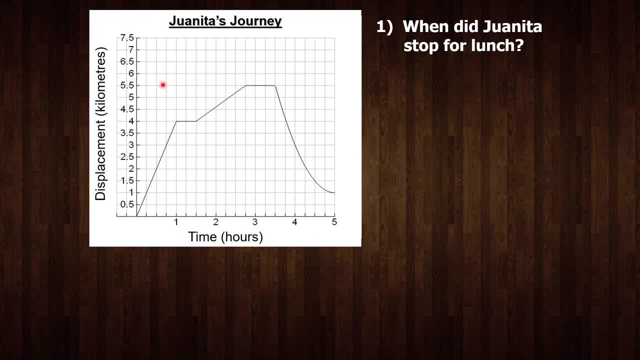 minute time interval where the displacement is 5.5 kilometers and it doesn't change. Now, remember she stopped twice: Once for lunch and once to watch a movie. So this one must be where she stopped for lunch and this must be where she stopped to watch the movie. So right here we have the displacement. 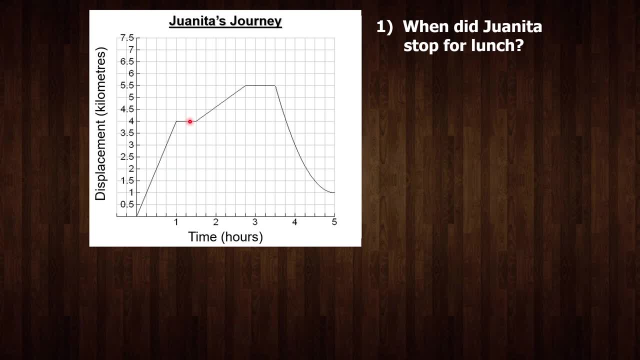 Here. we could say that one hour after leaving home is when she stopped for lunch, And, once again, that's because the displacement is constant there. It's staying at four for half an hour Next up. when did Juanita walk the fastest? Now, how are we going to figure this out? Well, once again. 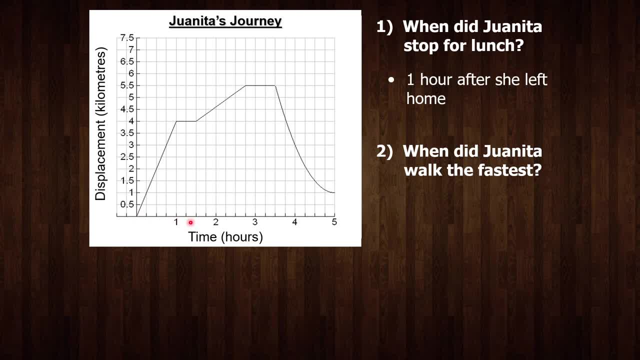 we're measuring displacement on the vertical axis and time on the horizontal axis, And let's take a look at the first parts of the journey where Juanita is moving, Starting with this one here. Notice that in this part of our graph, here in 15 minutes, we have Juanita moving one kilometer. 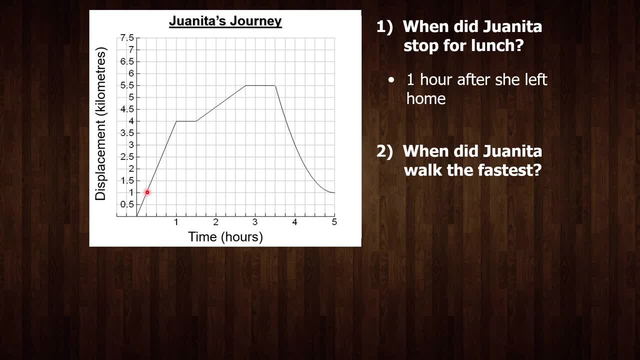 Okay, we can use that to come up with a speed. It would be actually four kilometers per hour, and we'll talk a little bit more about how we find that speed later on, But for now, notice, in 15 minutes she's moving one kilometer. Now, if we go to this part of the graph and look at how far she, 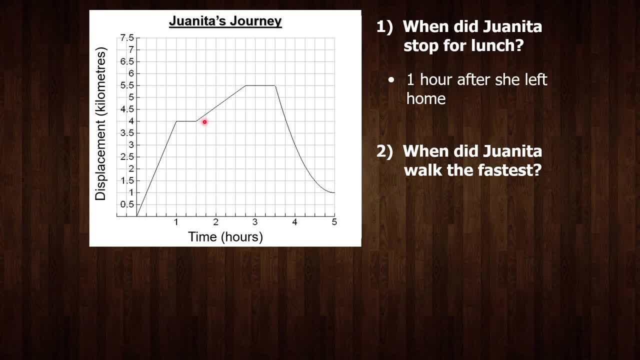 moves in 15 minutes. so that's one square. horizontally it is not one kilometer And in fact it's not even half a kilometer. So down here, 15 minutes, one kilometer movement. Up here, 15 minutes, less than a kilometer, less than half a kilometer. So she must be moving faster here Now. 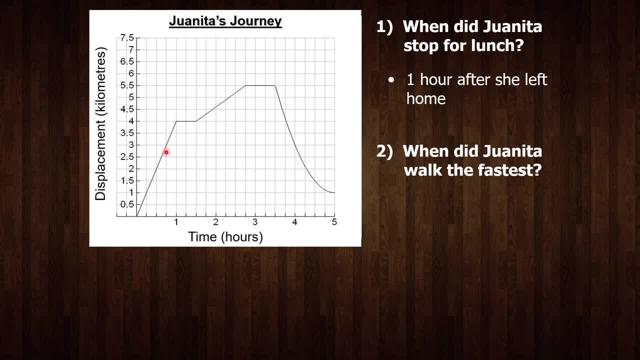 does that mean that the steeper segments on the graph always imply faster movement? Well, the answer is yes. Okay, for that reason, in a fixed amount of time, more displacement is being covered. Is this the steepest part of the graph? And the answer is no. We can see over here and now this: 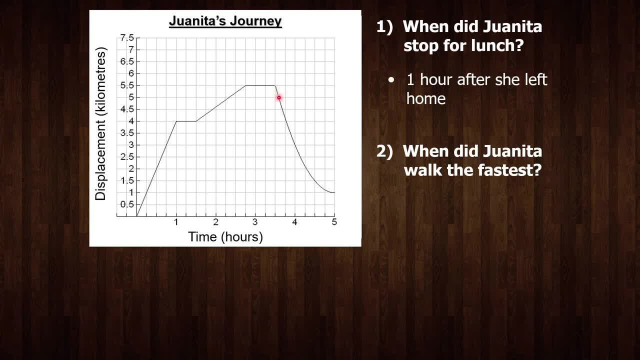 would be when she's heading home, because her displacement from home is now decreasing, which means she's getting closer to her home. But notice that in 15 minutes she travels more than one kilometer. So right up there, in that area, there would be the fastest. 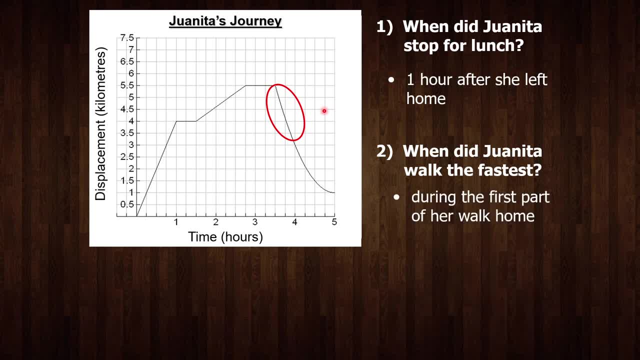 part of her journey, and that's when she's on her way home. Okay, just at the beginning, though, because that doesn't stay the same. Notice we have a curve segment here, and we'll talk about what that means a little bit later on. How long was the movie? Well, we've already talked about that, Notice we? 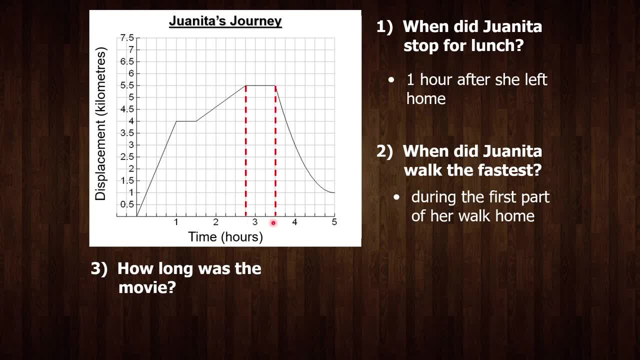 from the 2 hour 45 minute point to the three and a half hour point- that's where she was stopped for the movie- and that is a total of 45 minutes. Next question: when was Juanita's maximum distance? sorry, what was Juanita's maximum distance from home? Well, her maximum distance. 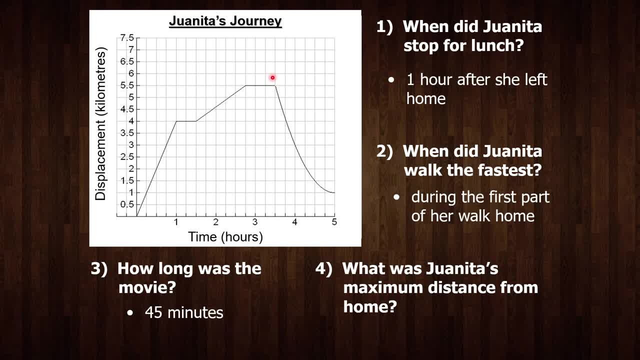 from home would be shown as the greatest displacement on our graph and we see that that is right up here and that's a displacement of 5.5 kilometers. so that is her, her maximum distance from home: 5.5 kilometers. Okay, moving on, At what speed did Juanita walk to the movie after? 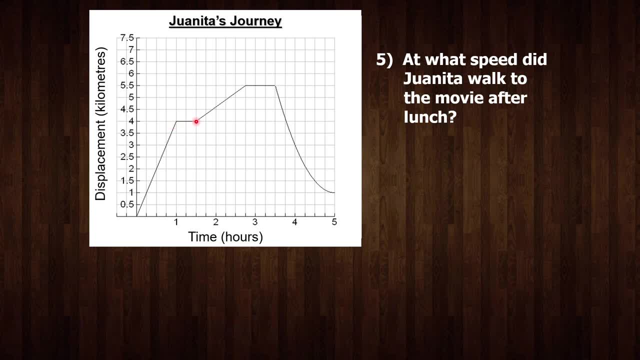 lunch. Well, we know that she walked here stop for lunch and then after lunch she walked to the movie. Now we want to follow the Friedrich Planck采es investigation structure. so let's start with the Pine Weather. I memories Going back over here in Rome. 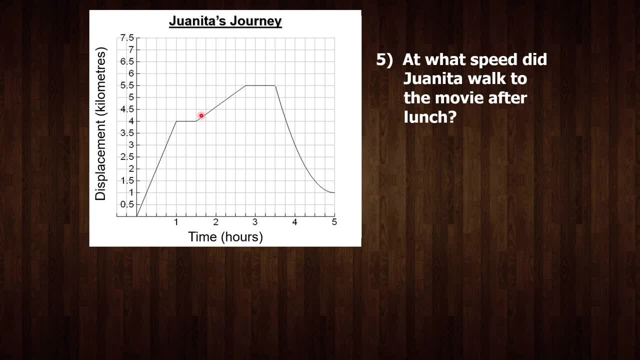 Well, we know that she walked here stop for lunch and then after lunch she walked to the movie. Now we want to follow the Friedrich Planck采. We want to find the speed at which she walked to the movie. Now, how do we measure speed? 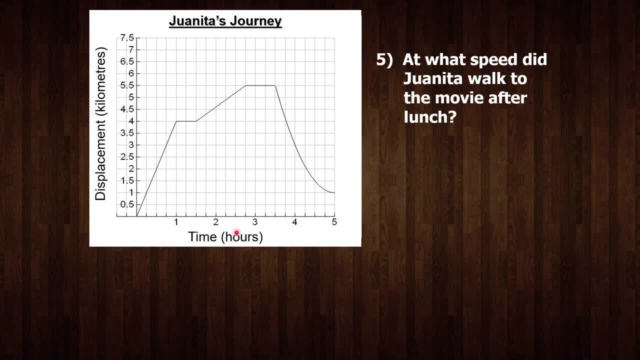 Well, we're measuring displacement in kilometers here and we're measuring time in hours here. So if we look at this part of the graph, we want to find out how many kilometers per hour she is traveling. Now. how can we do that? 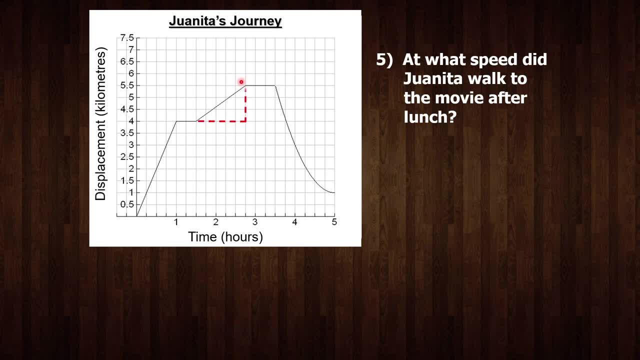 Well, we're essentially going to find the slope of this line segment here and we'll use the points at the beginning and end of the segment. Now notice that we have a 1.25 hour interval here. right, It's five squares and each square is 15 minutes. 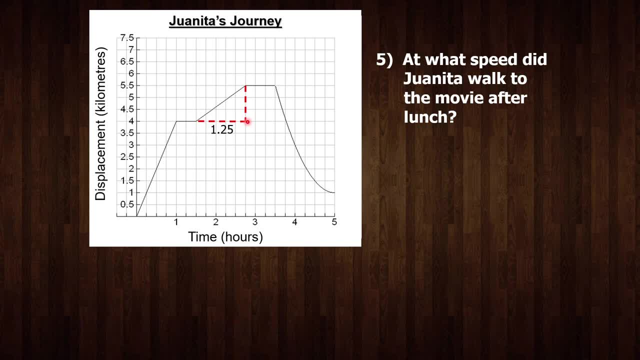 So you could say that's an hour and 15 minutes, but we want this expressed in hours, so 1.25 hours. Now, how much displacement do we have in that 1.25 hours? One and a half kilometers, okay. 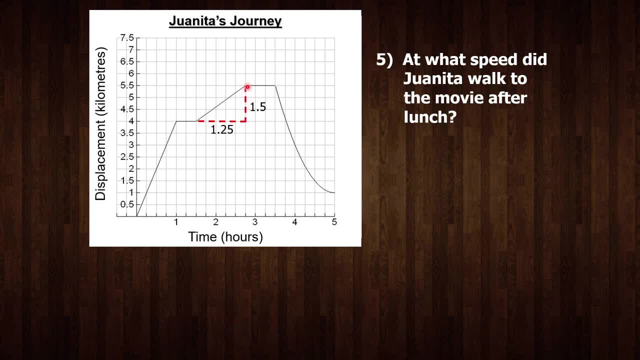 Notice here, two squares is one kilometer, so three squares here is one and a half kilometers. So she traveled one and a half kilometers in 1.25 hours. Now if we want to find the number of kilometers per hour, we need to divide. 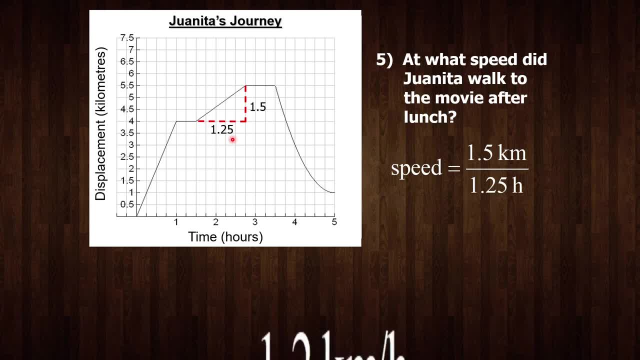 1.5 kilometers divided by 1.25 hours gives us the number of kilometers per hour, which is 1.2 kilometers per hour. So that's pretty slow. So does that mean if we want to find speed using a displacement time graph? 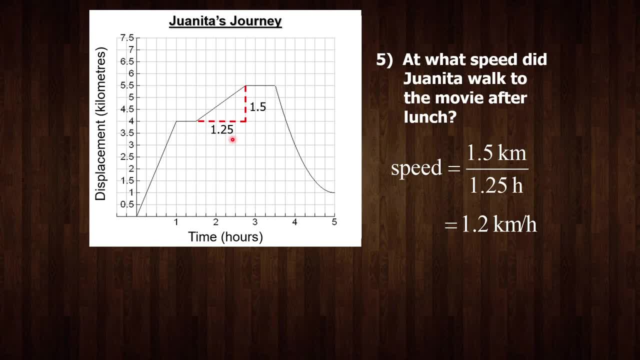 or you know, velocity, using a displacement time graph, we can just find the slope, We can just find the slope of a segment, and the answer is yes, provided that in this case, as in this case, we have a straight line segment. 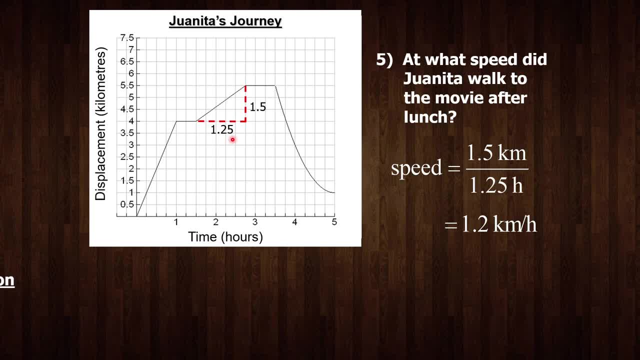 And we'll talk later on about what happens when we don't have a straight line. Finally, some questions for discussion. What other information does this graph tell us? Well, I'll draw your attention to this part of the graph right here. Notice that it starts off quite steep. 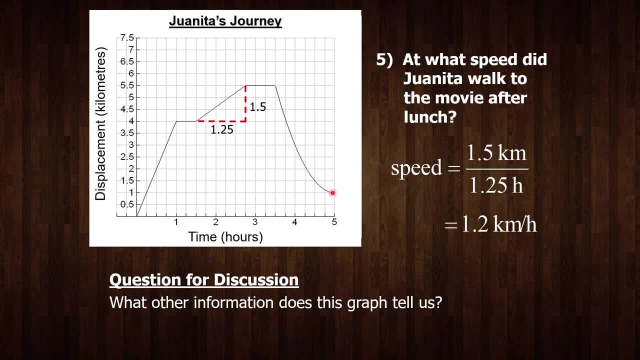 but then it gets less and less steep as we get closer to the five-hour point. Now, what does that mean? Well, the steeper that the graph is on a displacement time graph, the faster the motion is, and that is what's happening here. 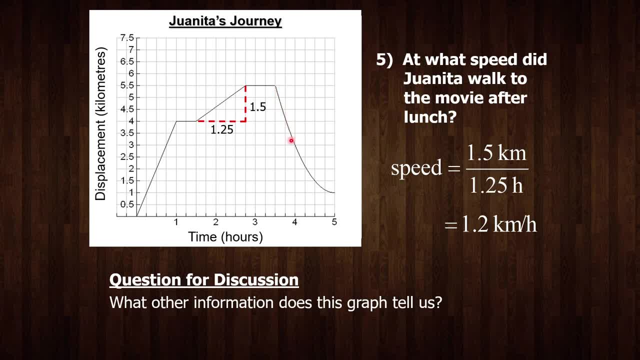 We have fast motion because it's quite steep, but then, as it gets less steep, that must mean that the speed is decreasing. In other words, Juanita is slowing down. Now you might ask: why did Juanita slow down so much here before she got home? 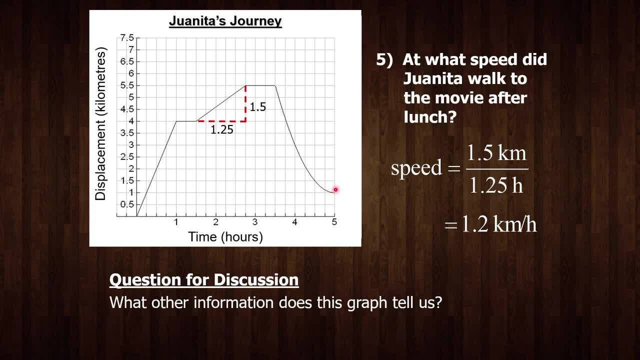 Notice she didn't make it back home. I'll let you think about why that might be. One other thing that I'll mention before we wrap things up here is to think about how realistic is this graph at describing somebody's journey if they're walking now? 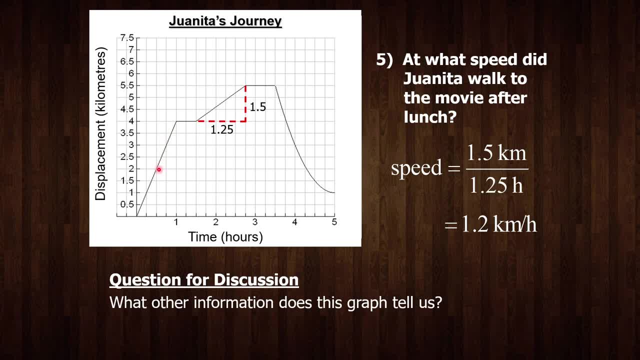 What do I mean by that? Well notice, she was traveling at four kilometers per hour at this point, and then, instantly, she was stopped. Now, is that possible to go from a speed of four kilometers per hour to zero kilometers per hour in an instant? 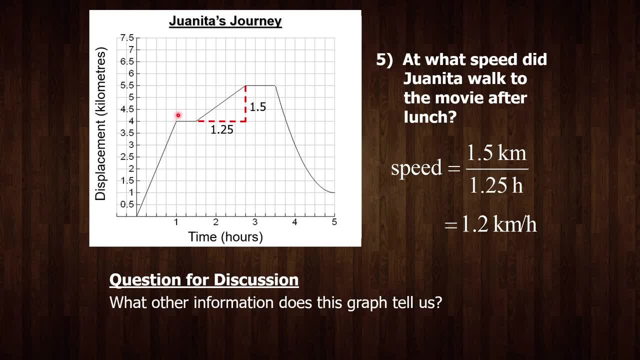 And I think you'll realize that no, that's actually not possible. She'd actually have to slow down, Even if she slows down very quickly. So what I'm getting at is that this sharp corner here is not very realistic. What we'd really probably see in real life is a kind of a curve.